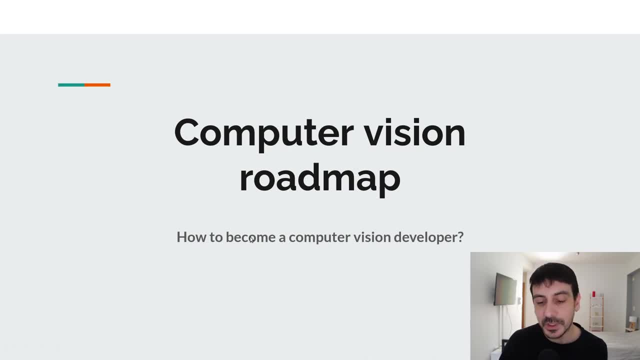 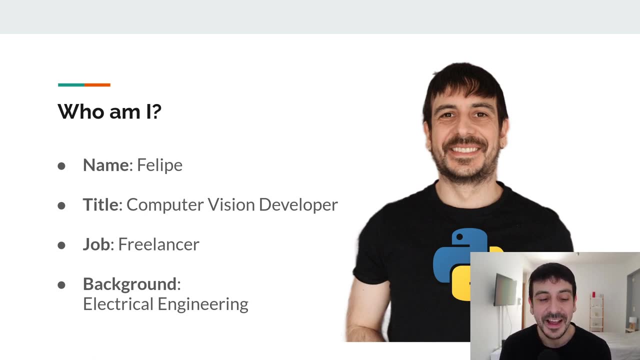 going to show you in this video. Remember, we are going to answer the question how to become a computer vision developer. The first thing I am going to answer in this roadmap is: who am I? And this is a very quick, overall, high-level description of who am I. My name is Felipe. 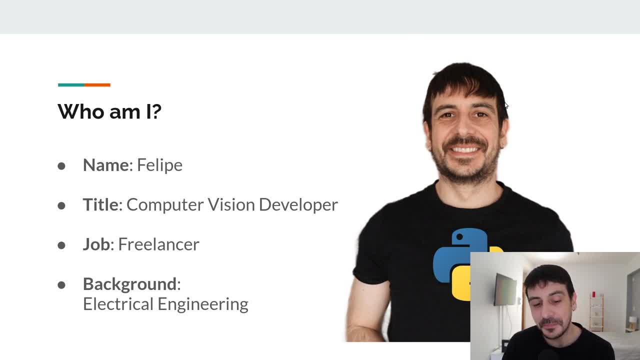 I'm a computer vision developer, and this is me. This is a picture of me. I work as a freelance developer, as a freelance contractor, and my background is in electrical engineering. So that's a very, very high level description, a very quick introduction of who am I. Now let's continue. 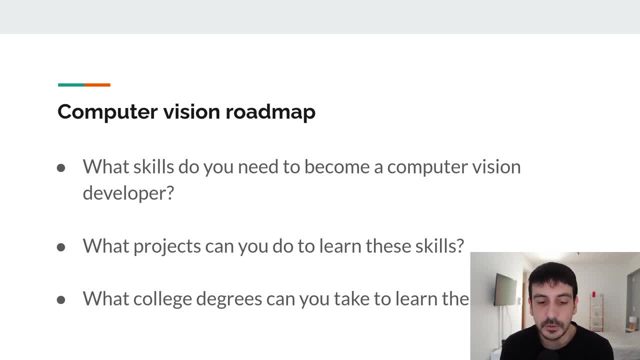 This is the computer vision roadmap we are going to cover in today's tutorial. in today's video, I am going to answer these three questions: What skills do you need in order to become a computer vision developer, What projects can you do to learn these skills And what college degrees can you take in order to learn these? 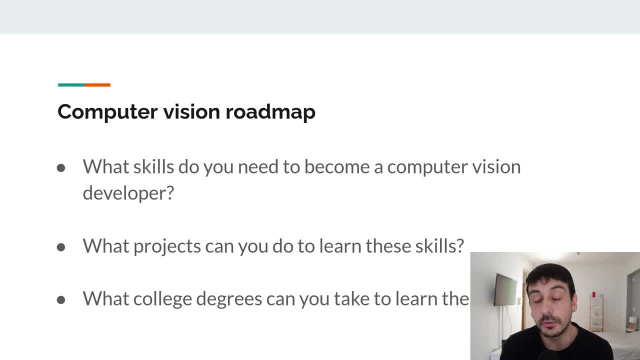 skills. There are people who prefer to learn on their own, taking projects and working on their own, And there are people who prefer to take college degrees. So I am going to talk about all the different skills you should acquire in order to become a computer vision developer. 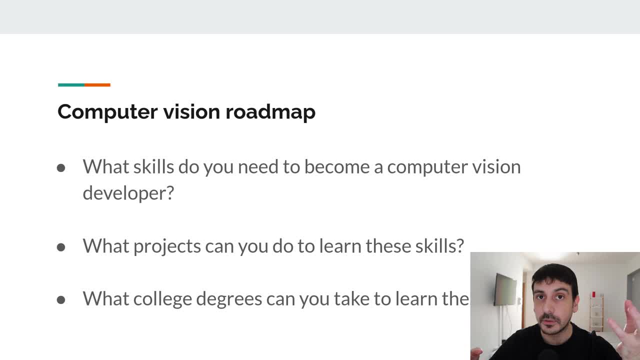 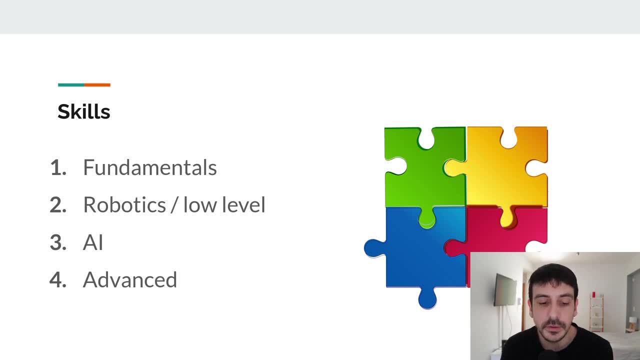 and all the different ways you can acquire these skills: Taking projects on your own or taking college degrees. So let's continue, And I have organized all the different skills you should need to learn in order to become a computer vision developer into these four different modules. The first module is about 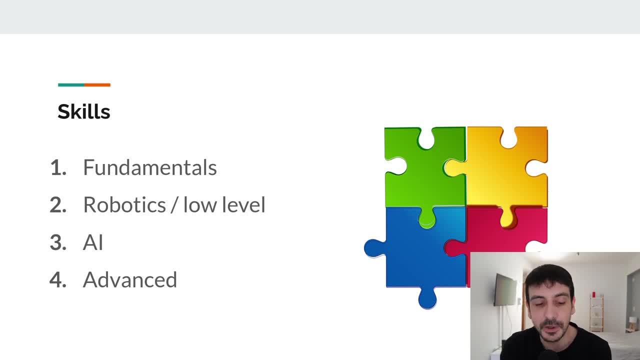 all the fundamentals, all the foundations you need to learn in order to become a computer vision developer. Then a second module is about robotics or low level programming. Then the third level is about artificial intelligence, about AI, And then the fourth module, which is the module for all the 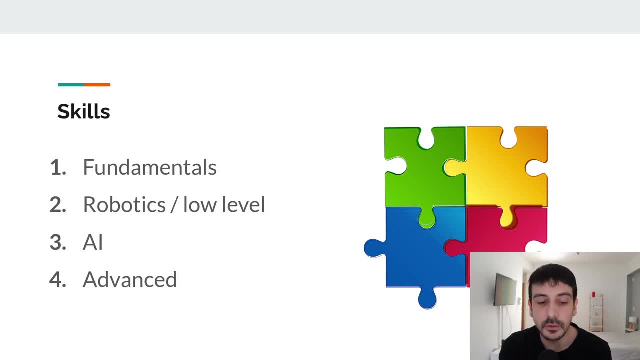 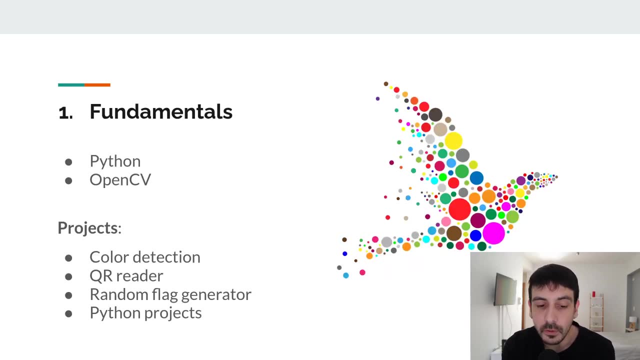 advanced topics for all the advanced skills you need to learn in order to become an awesome and super expert computer vision developer. So let's start with it. The first module, which is the fundamentals, the foundations. it's basically Python and OpenCV, And this is 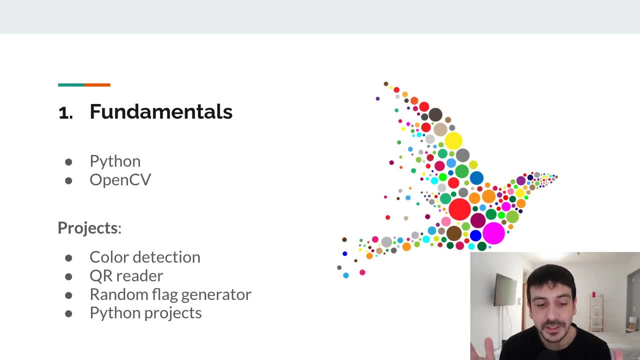 by far the most important module of all. It's amazing how many problems you can solve using only Python and OpenCV, And I will say that 70% of absolutely all computer vision problems can be solved with Python and OpenCV only, without using any other computer vision algorithm or 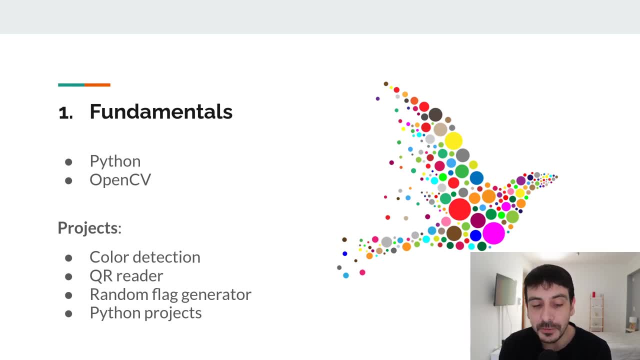 technique or something more complex. Only by using Python and OpenCV you will be able to approach at least 70% of all problems. So this is basically- this is definitely the most important module of all, And these are a few projects that are going to give you the skills you need in order. 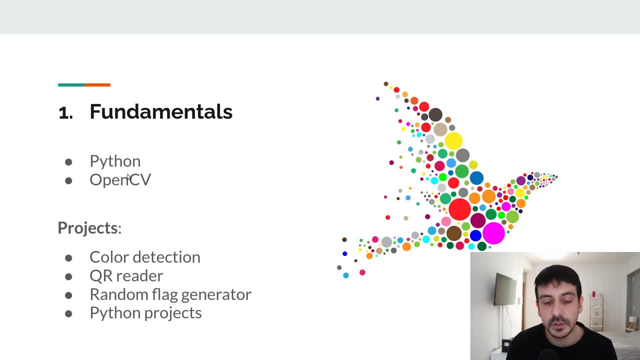 to learn Python and OpenCV, And some of these projects are some of the previous videos in my channel. For example, one of my latest videos is about color detection. you could work on a QR reader. you could work on a random Flags generator, for example, this one of my previous videos. 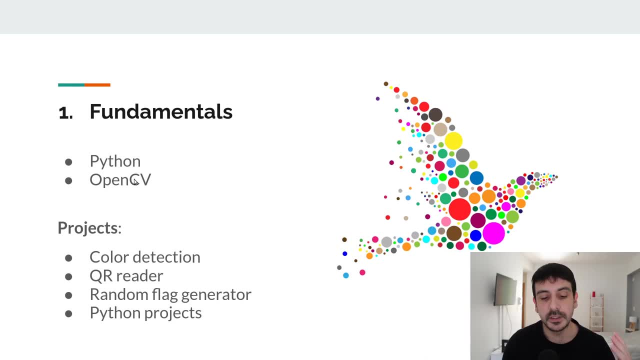 This is also a very good project in order to learn Python and OpenCV. In this video, I show you how to create random flags by using Python and OpenCV, And it's basically it's only about shapes. So you start with a rectangle and then you create shapes on. 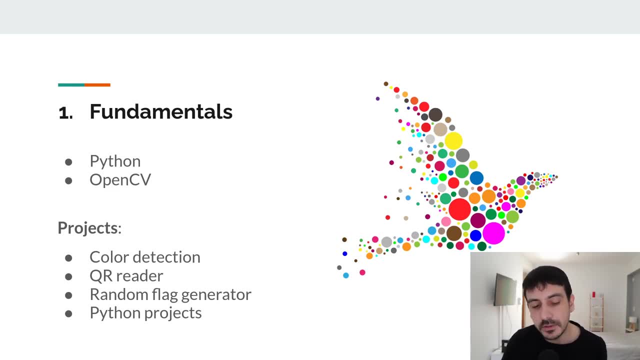 top of this rectangle And the internal expressions, and this is how you will be able to create these and then you create overlays. so it's definitely a very good project in order to get more familiar with shapes and overlays and so on, and randomness and a lot of randomness, and you can also take 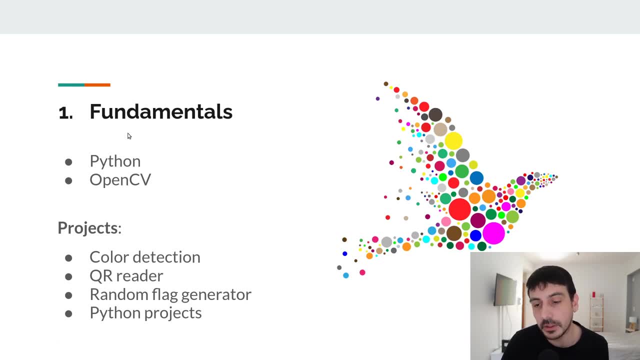 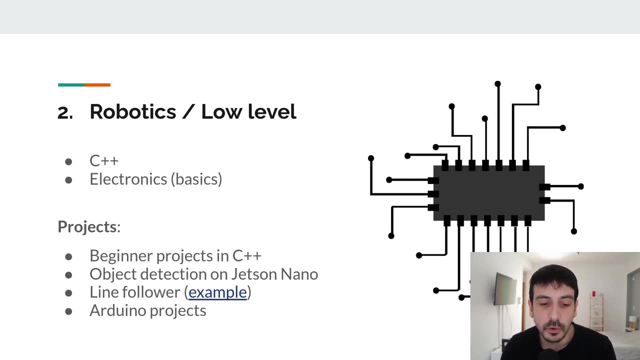 absolutely any other python projects because it is about learning python. you don't really need to learn python through computer vision. you can just learn python taking absolutely any project. then the second module is about robotics and low level programming. this is where we have c++, which we all know. it's a very common language, programming language for working with computer. 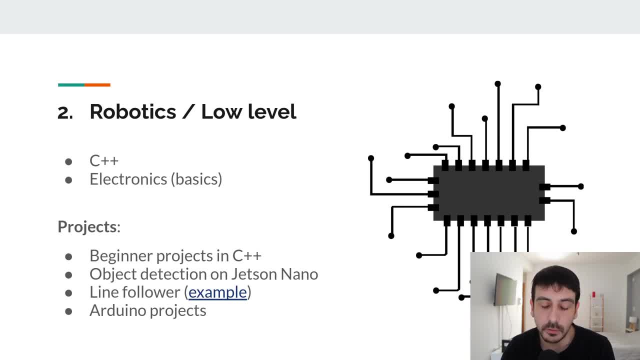 vision. basically anything you can do with top ncb in python, you can also do top ncb in c++ and also electronics and some basic knowledge of electronics, because if we talk about electronics we can go super, super complex, we can do some very crazy stuff and we have many different. 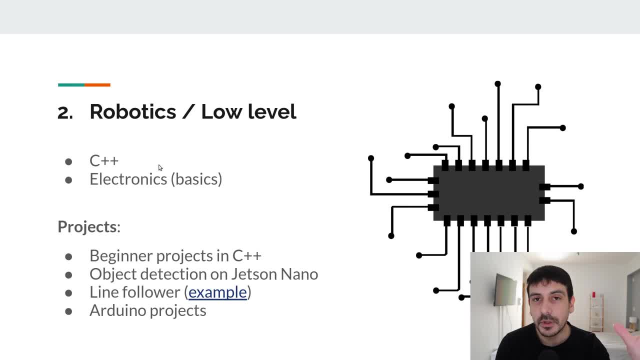 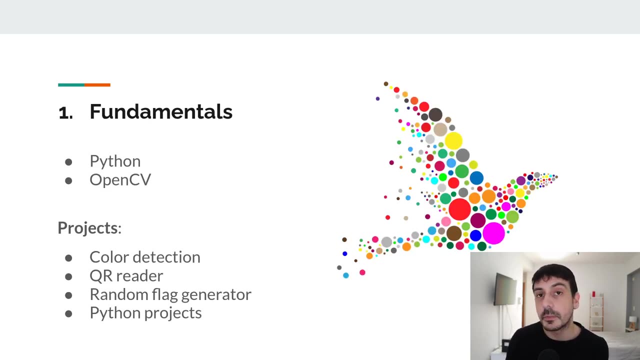 possibilities, but i'm talking about some very you, the the basic of the basics of electronics, the foundations of electronics, and some of the projects which are definitely going to help you to acquire all of these skills. c++ and electronics are some beginner projects. in c++, for example, all the projects i have mentioned in the fundamentals. 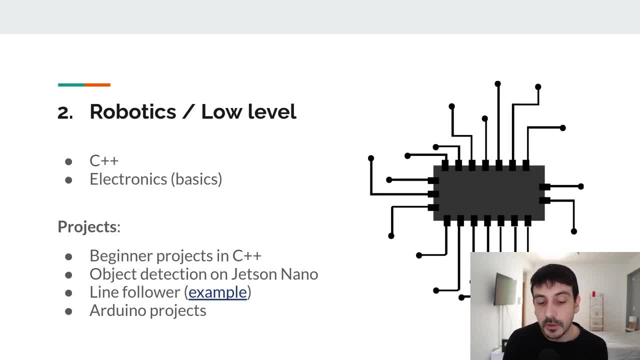 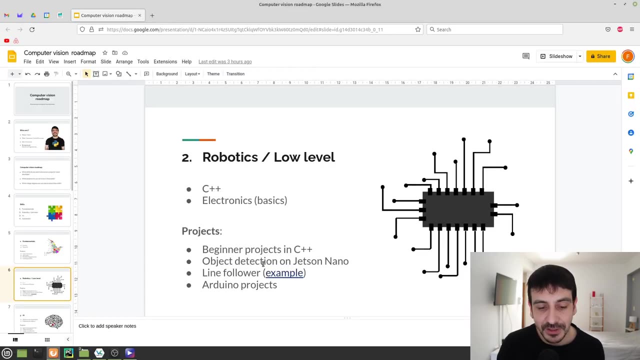 module, but in c++. then if we are talking about edge devices and doing our inference on an edge device, we can work. we can take a project of doing object detection on a jetson nano. that's a very interesting project. we could work on a line follower and that's a very, very interesting project. let me show you exactly what i mean with a line follower, in case you are not familiar with this type of. 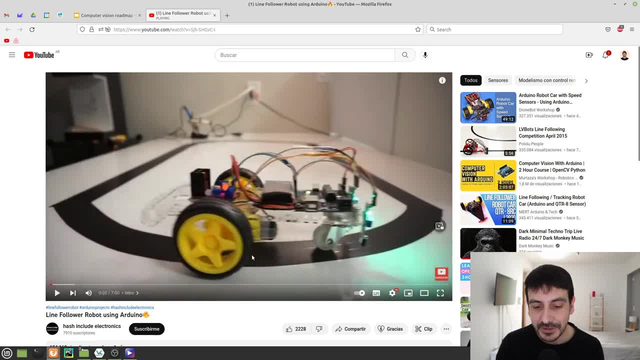 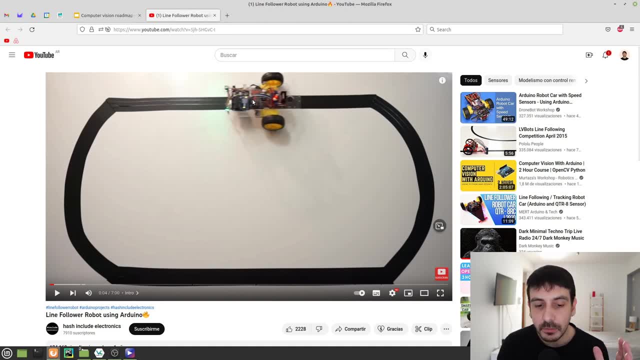 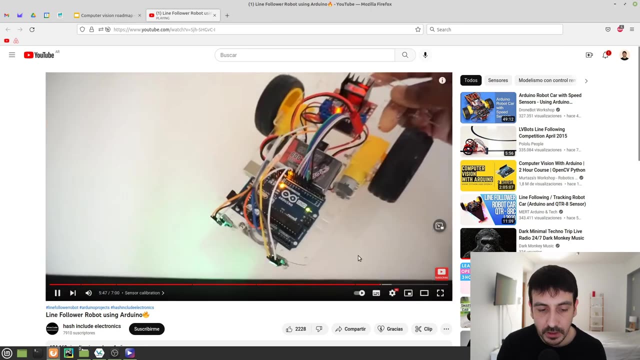 projects, or with robotics, uh, projects- working on a line follower. it's doing something like this: where you have a robot, where you have something like this and you have, and you, you need to make these robots to follow a given line. so let me show you. this is a little more clear and the idea is that 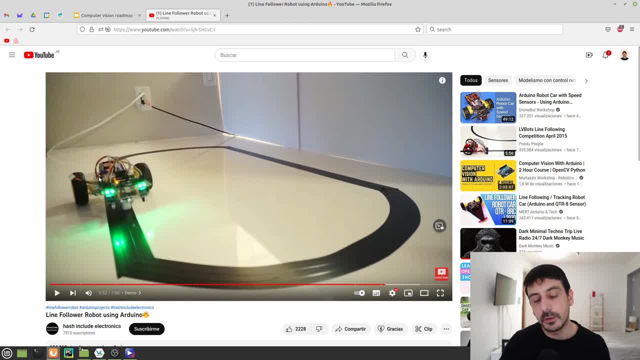 you are going to have something like an arduino or a chest of nano or whatever, and you are going to have some sensors. so the idea is that you are going to be able to read the color you have like right in front of you and, depending on that color, you know that if you are following the line or not. 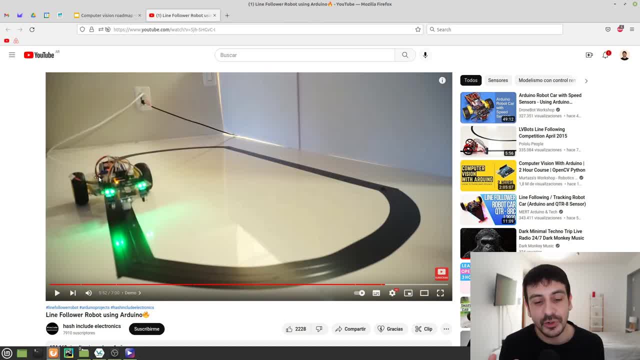 and although this sounds like a very simple project and a very easy project, trust me that it's not as simple as it sounds. the one thing about taking these projects is that you realize that, for when you are programming something that's on an edge device, that's like robotics- 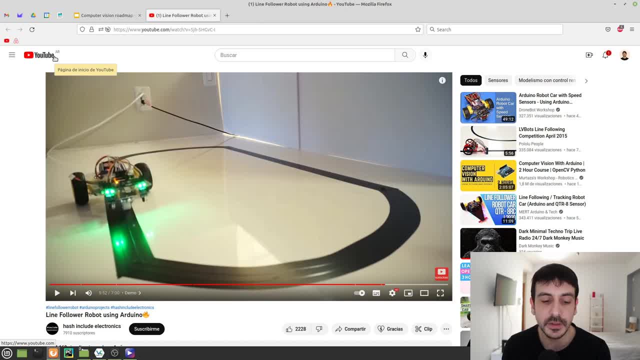 that's like a real device, like an actual device, like physical device, then you need to adjust your programming. you need to adjust the way you think about problems, the way you approach problems, because i can promise you that it's not going to be exactly the same as if it's only like a piece. 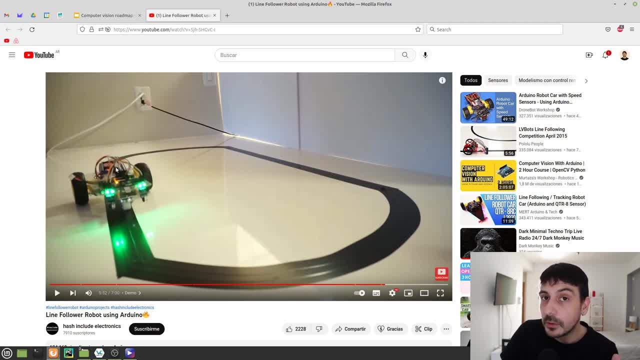 of code which is running on python on your local computer, because when you are only familiar with software, the way it usually works is that you have something like a script or a piece of code and if you execute that script or that piece of code once and again, you 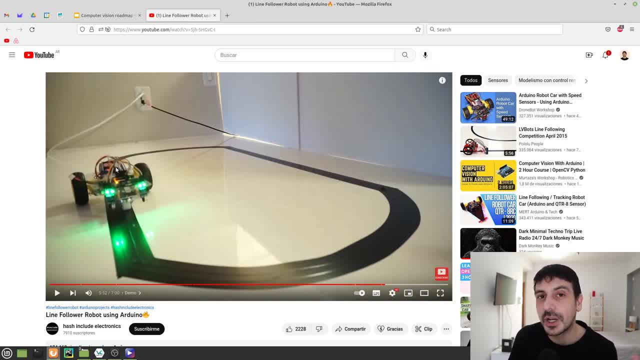 are always going to have pretty much the same result. that's pretty much how software works. but when you are working with a real device, with a physical device, it could happen that you are executing the same script, the same code once and again and it could happen that every time you have 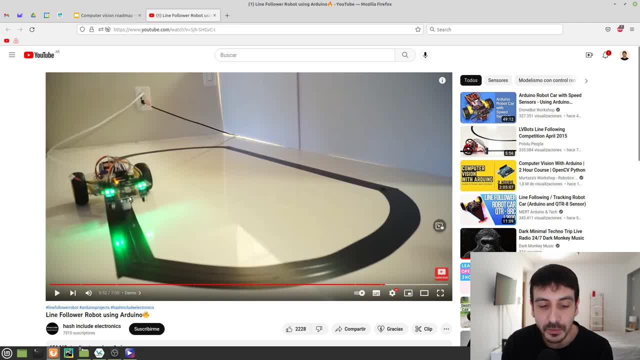 different results, because if you are measuring the color, for example- in this case, i don't know- maybe the lighting changes, or maybe you have a lot of noise from your sensors, or maybe something happens, and, yeah, you get the idea. so everything is going to be slightly different, as if you were only 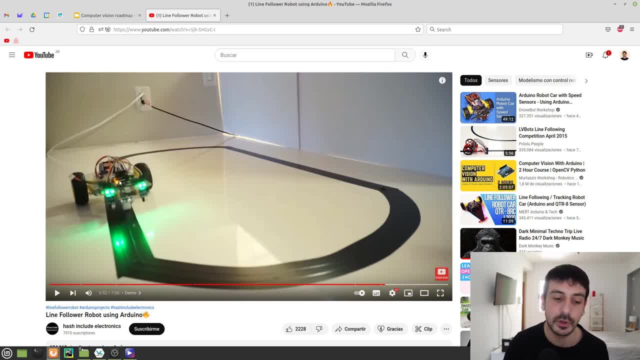 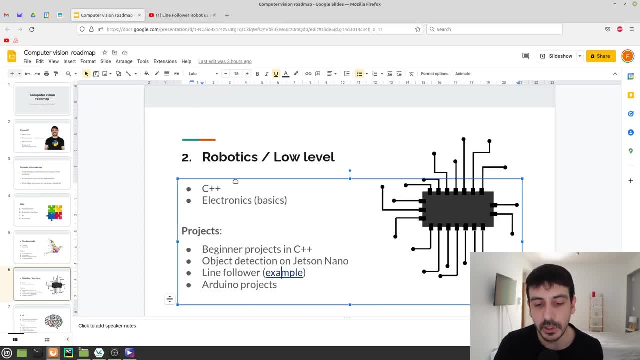 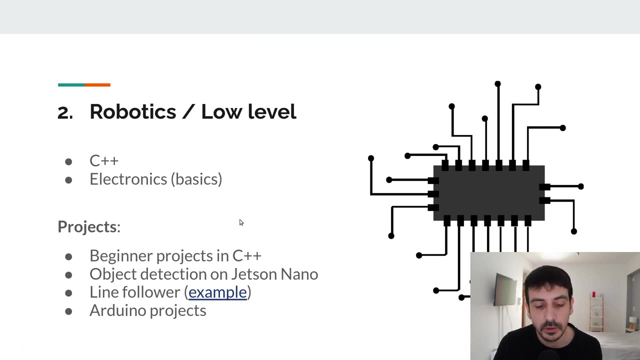 programming like a piece of software which is going to be running on your local computer. so this is definitely super important and super valuable in order to become more skillful in learning how electronics works, or the very the basic, the basics of how electronics works, and also you can take any other. 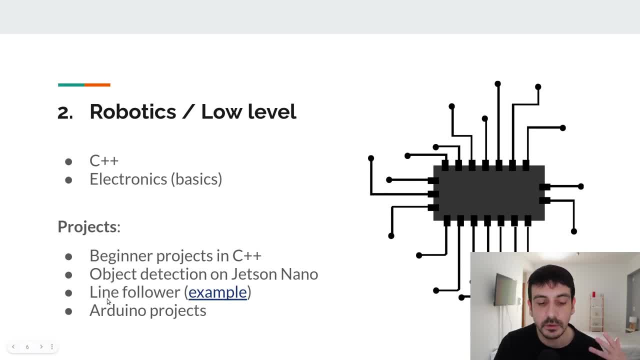 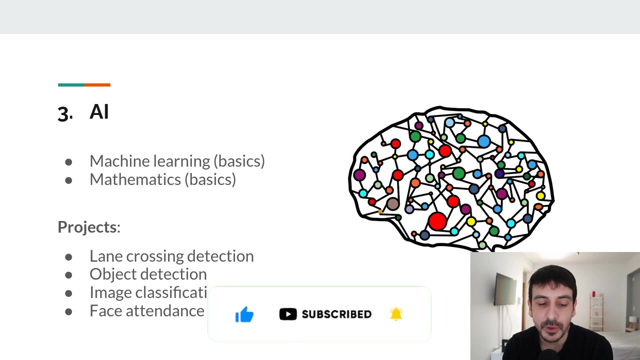 Arduino project- basically, absolutely any Arduino project- is going to give you the intuition on how to work with robotics and with a low level programming, or how to. what are they? how to approach those projects? it's basically how to approach a project involving electronics, so let's continue then. the third module is about artificial intelligence, or AI, and this is where you are going. 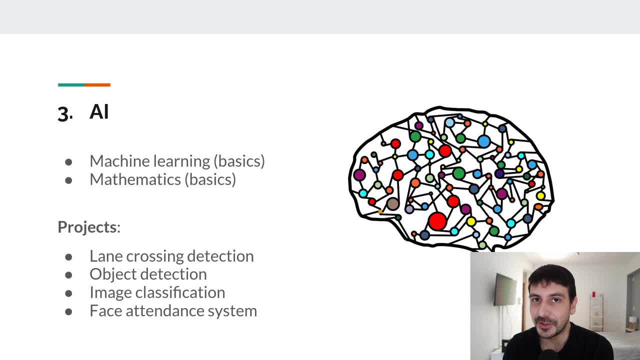 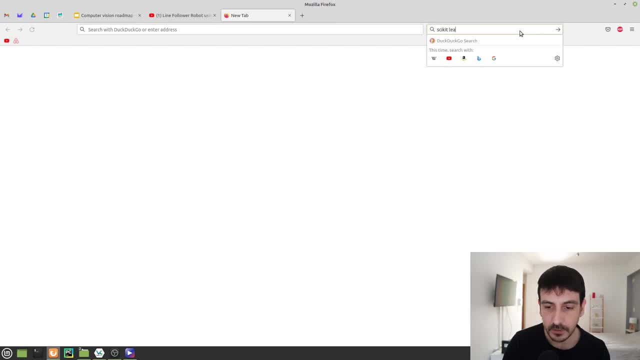 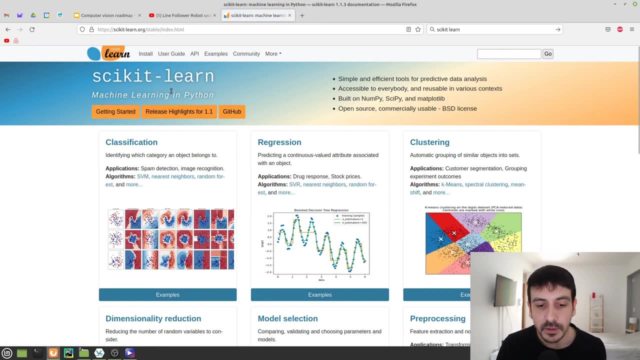 to learn machine learning and mathematics and the very basics of machine learning and mathematics and specifically, the idea is learning this library, which is a very popular library in python in order to do machine learning, which is called ckit learn, and with this library you can do pretty much anything you want regarding machine learning. you can do image classification. 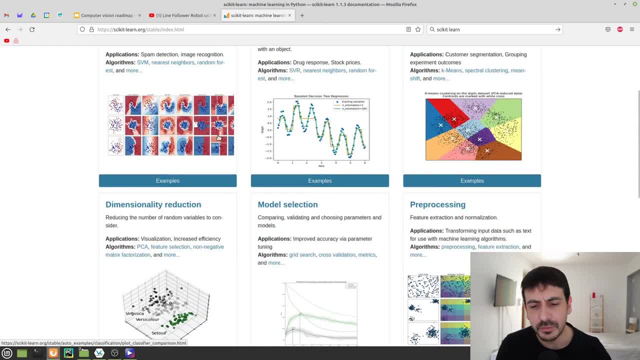 you can do regression, clustering, you can do pretty much anything you want. you have different dimensionality reduction, as PCA or also other techniques can do that. data pre-processing, so you can adjust your data in different ways: in order to clean your data, in order to or in order to make it nicer, in order to input this data into a classifier. 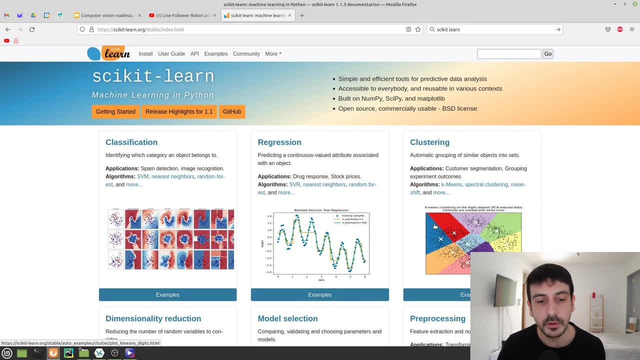 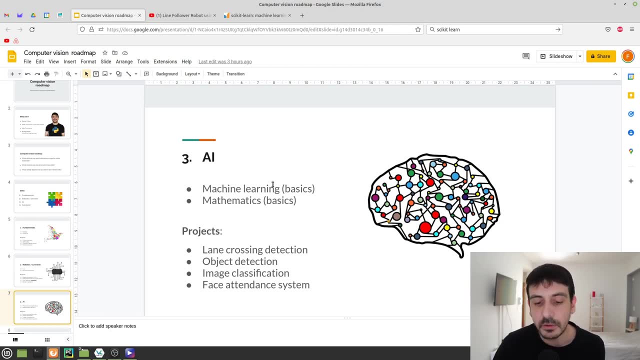 so you can do pretty much anything you want. this is a very, very comprehensive library and this library which is very commonly used in machine learning projects. so when i talk about the basics of machine learning, i'm talking about everything that you can do with SQL Learn. that's pretty much. 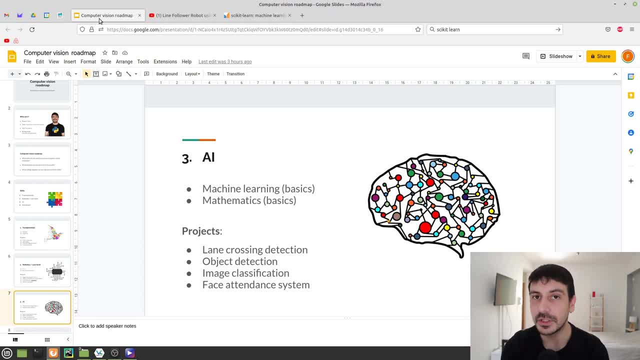 the idea it's SQL Learn and also some image classification and object detection, which are the most important fields of computer vision, right? so everything that's like building an image classifier or building an object detector or anything you can do with SQL Learn, that's pretty much the idea. 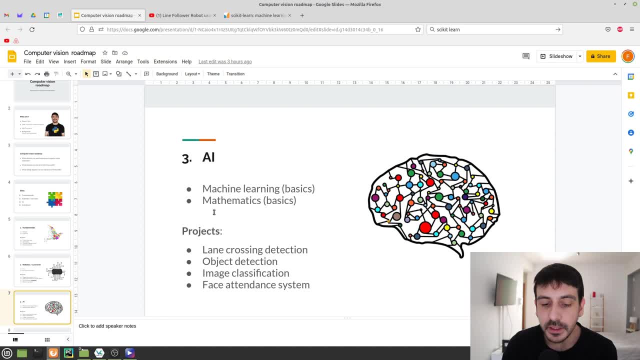 of what i'm talking about when i'm talking about machine learning basics, and then, if we talk about the basics of mathematics, i'm talking basically about geometry or everything that's like space, spatial mathematical notions or something like that. I'm going to show you an example, which I 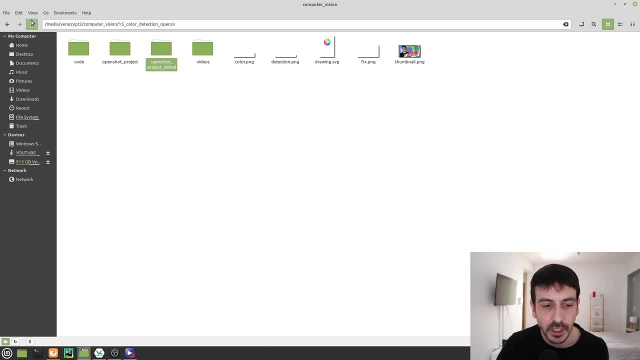 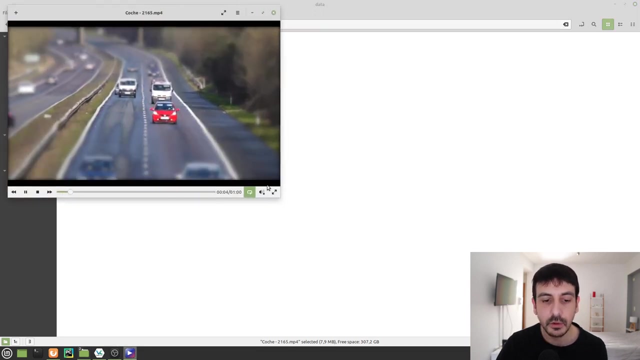 think it's a very good example of what I mean when I say basic mathematics, and this is regarding one of my previous videos with the lane crossing detector. Let me show you a video which is a video I used for this detector, and in this video I show you how to detect a lane crossing using this. 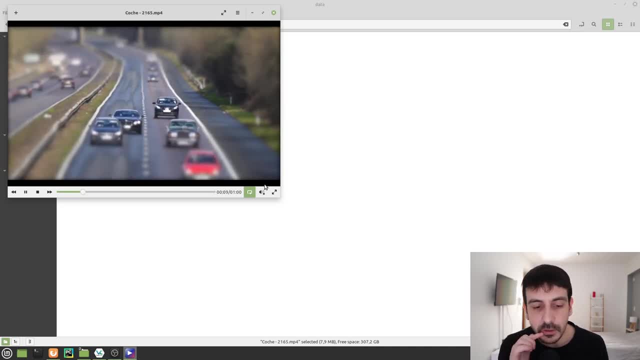 video and the thing about this video and I think about this project and the way I think this project is pretty much related to what I'm talking about, this basic knowledge of mathematics- is that the way I approach the solution of this problem is dividing all this frame, dividing absolutely. 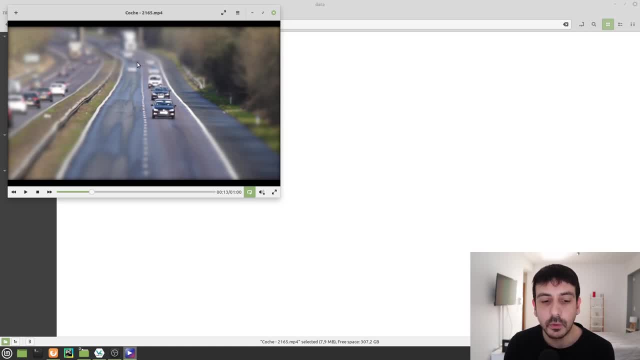 everything we are seeing here into different regions. So we have a region for everything that's not the highway right, We have a region for the background. let's say, then we have another region for one of the lanes, then we have another region for the other one, the. 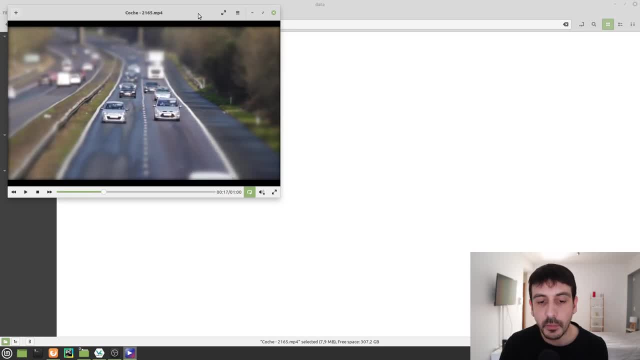 other lane. Once we have detected all the cars and we have all the environment, all of our environment, divided into different regions, it's super, super easy to detect a situation like this, like this lane crossing. I think we're going to see one right now. It's super, super easy to detect a situation. 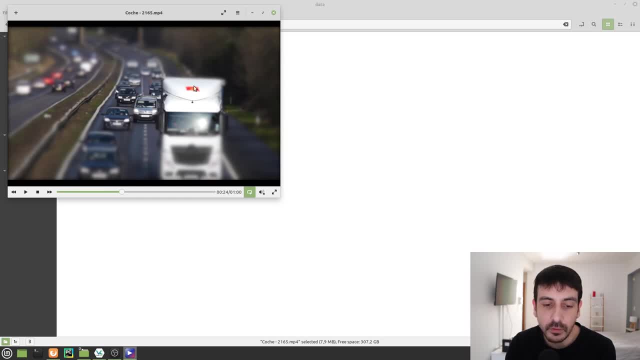 like this, because we have this as one of the regions, this as the other region, and then, once we have detected the car, it's just assigning a lane, designing a region for each one of our cars. Let me show you now this image, which is the. 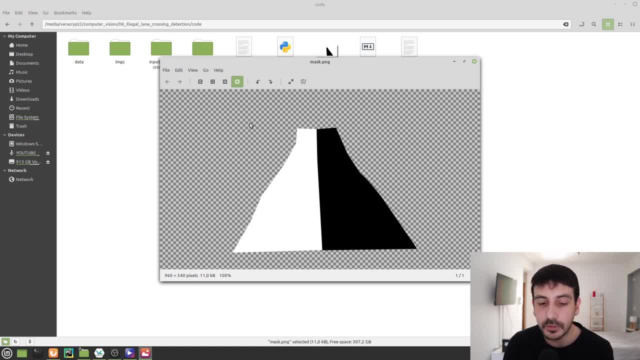 image I used in this video. This is exactly what I'm talking about. We have the background, which, in this case, is like transparency. then we have one of the regions in white which is one of our lanes, then we have the other lane in black and this is pretty much all. We have our 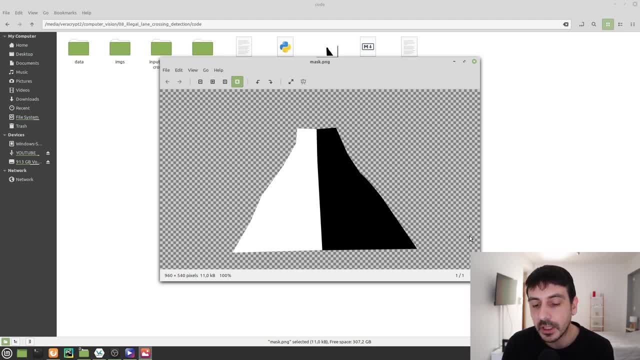 highway, which is these two lanes, and then we have everything else, everything else as our background, which is a transparency, And this is what I'm talking about when I say basic mathematics. This is what I'm talking about when I say something like geometry, or 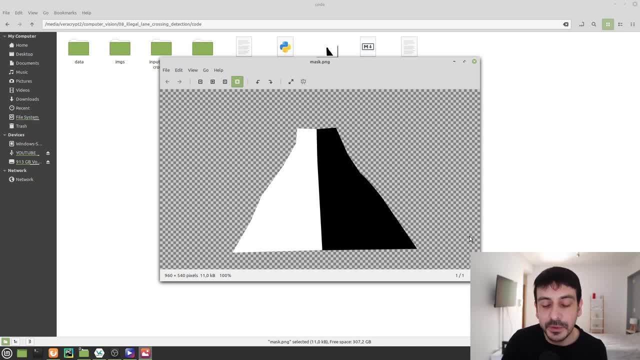 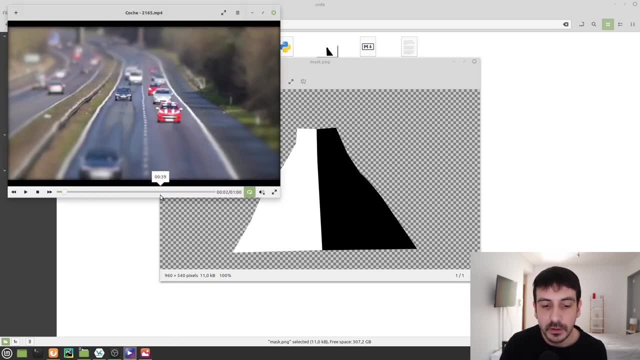 something like the spatial mathematical something- because as a computer vision developer you should be very fluent- to do something like this, right To divide all of your space, all of your environment, into different regions and to do different things with it. It should be like super. you should have a lot of intuition on how to do that. 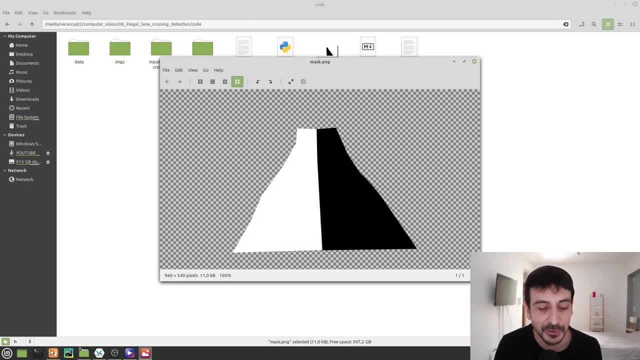 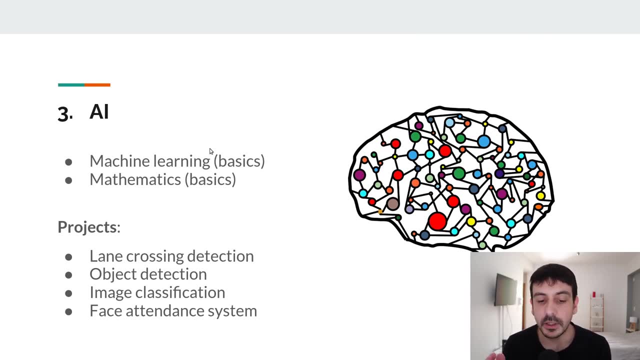 So knowing geometry is going to take you very, very far in computer vision, And that's why I created this slide with these two skills: machine learning, the basics of machine learning, So image classification, object detection and secret learn, and the basics of mathematics. 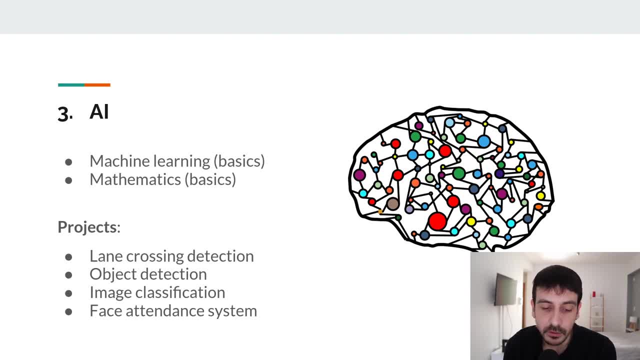 And some of the projects you can take are the, for example, the lane crossing detector I show you as an example, Then pretty much anything involving object detection, or pretty much anything involving image classification, or also another of my previous videos, which is building a face attendance system. This 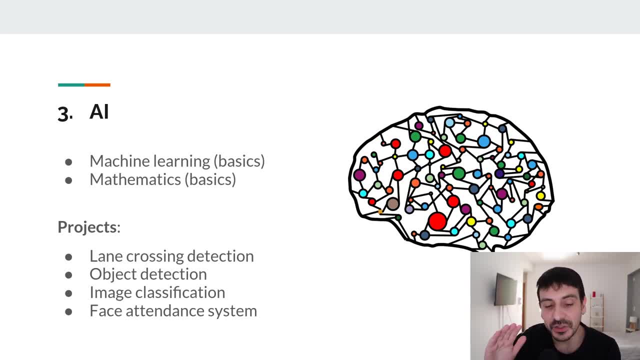 is like slightly more complex. more complex is pretty much like in the in the, in the limits of what, if it's basics or if it's more advanced, because we are not doing only face detection but we are also doing face recognition, which is like a slightly more. 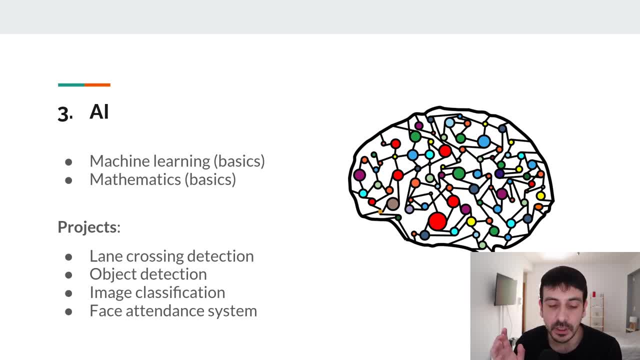 complex topic, But the way this uh face recognition is done, which is basically calling like a, like a library, something that's ready And it works out of the box. the way it works, you can just forget about all the complexity. 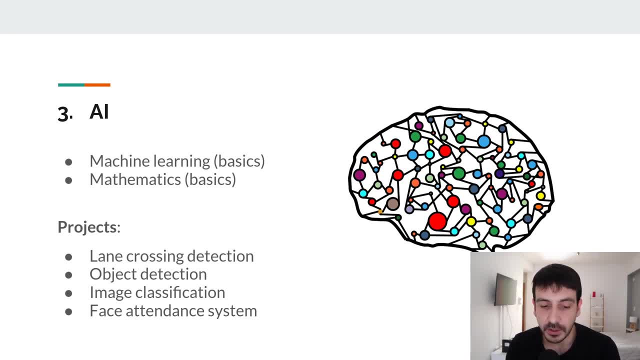 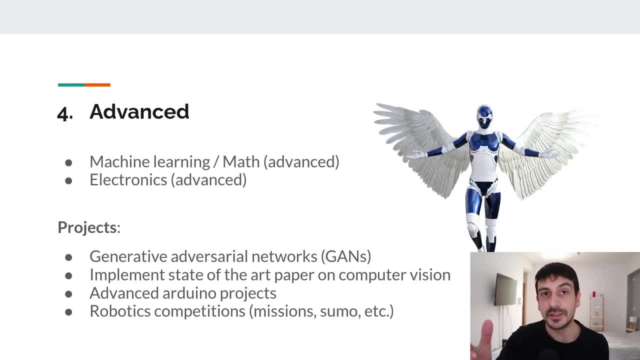 and you can just uh, run this project using, like you, some very, very basic knowledge of machine learning. So that's for this model, AI. And then let's move to the advanced model, And this is where you are going to learn, like more advanced skills on machine learning, more advanced. 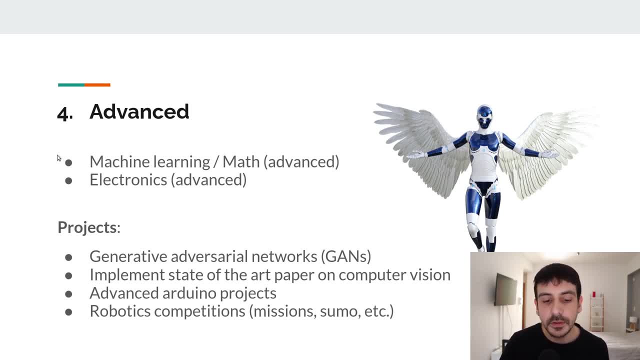 mathematics, more advanced electronics- all of these different skills are super, super, super important and so far we have only learned this skill, is these skills in a more basic level. in this module, the idea is to go super, super, super deep and to learn as much machine learning, as much mathematics and as much. 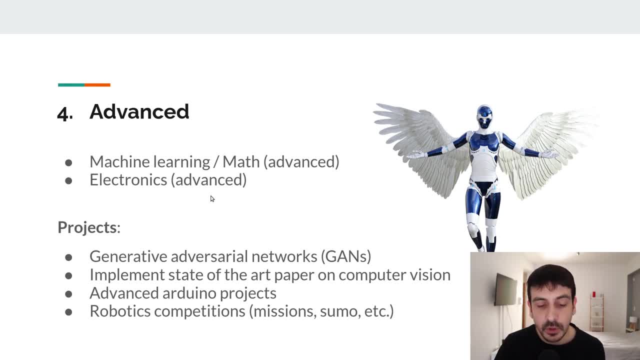 electronics as possible, and some of the projects which you can take in order to learn these skills in a more comprehensive, in a more advanced way are generative adversarial networks, pretty much anything containing gans, and this is a very good way to learn more advanced machine learning. 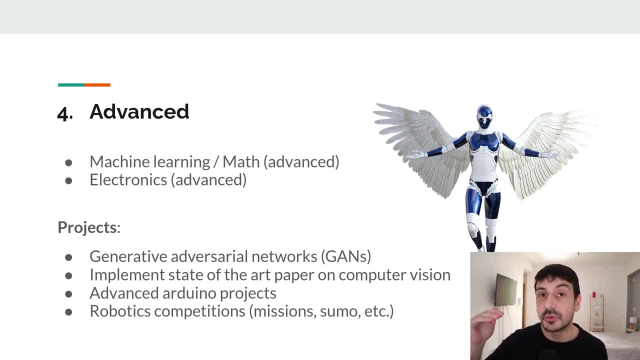 if you train a generative adversarial network again from scratch, from zero, then you will realize that it's slightly more complex than training an image classifier on an object detector. it's slightly more complex, it's going to be more complex. so this is an ideal project for learning, like more advanced machine learning or more advanced. 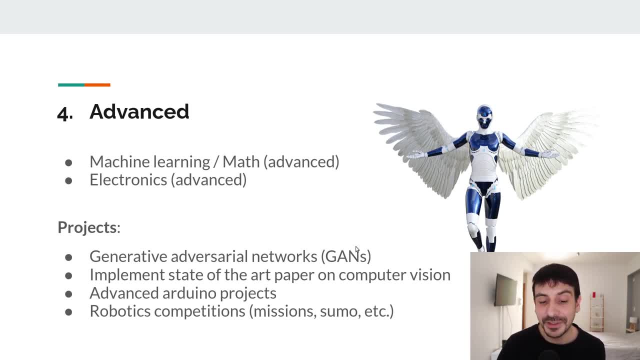 mathematics, and you can definitely do some very, very crazy stuff with GANs. so this is basically: this is a very good project. then another project you can take is implementing a state-of-the-art paper on computer vision. that's also a very good idea if we talk about state of the art in computer vision or machine learning. 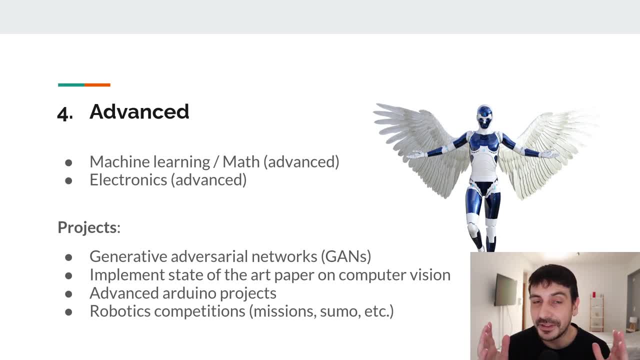 you are going to find some very, very noble, very crazy, very, very advanced stuff. then also in for the advanced electronics. you can take pretty much any advanced Arduino project. you can just search on youtube and there are many, many examples, or also some robotics competitions. and let me 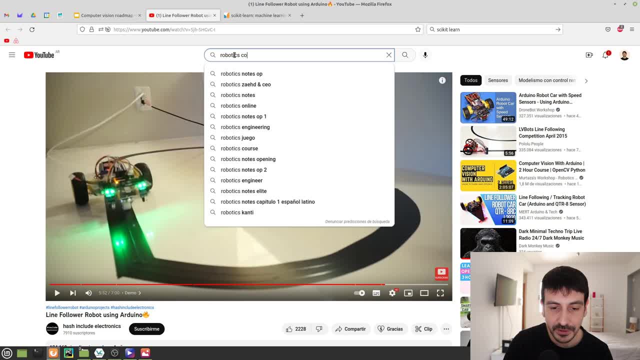 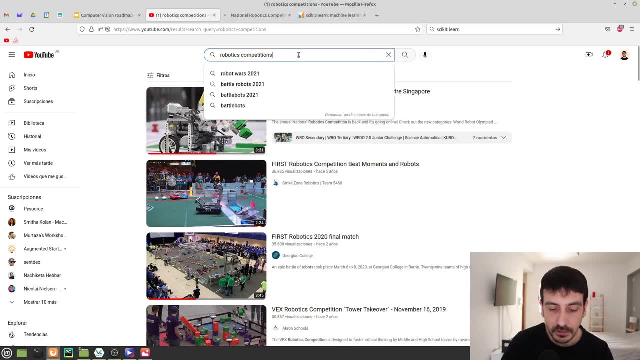 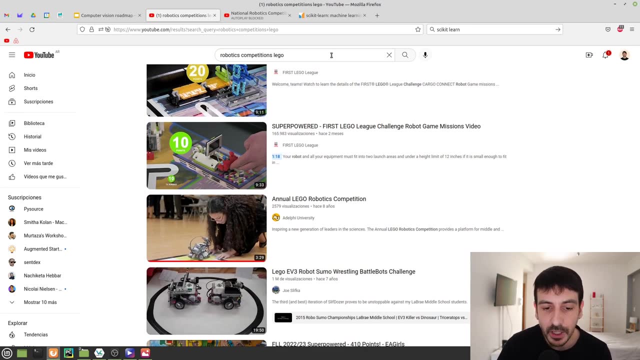 show you exactly what i mean. i'm going to search robotics competitions. this is a very good way to learn more, more electronics, because, uh, there are some of these missions, some of these competitions which you, you have something like a line follower, but your robot, your agent, needs to do some more complicated stuff, some more complex stuff. so you have something like: 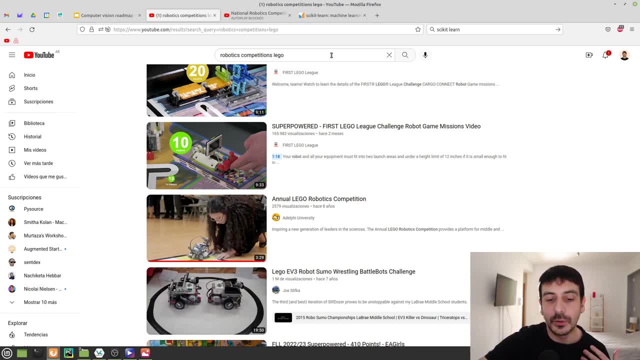 a mission, so you need to take something to somewhere or you need to do i don't know. you need to manage all many different sensors and you have a camera and you have, like, these are very, uh, these are very nice projects. i really, really enjoy them. i don't know if we are going to have 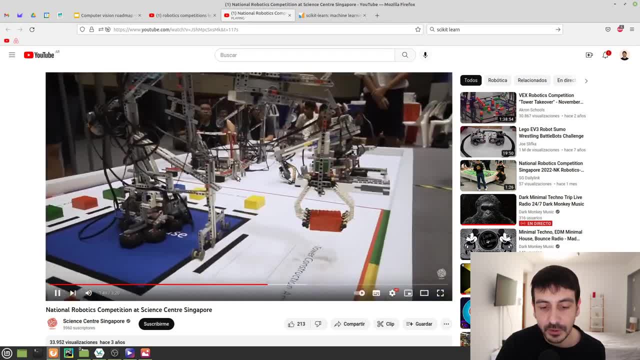 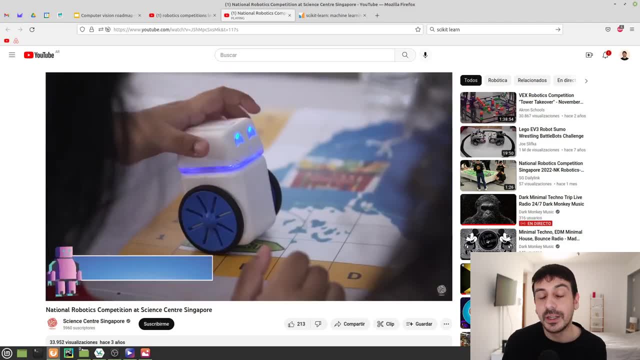 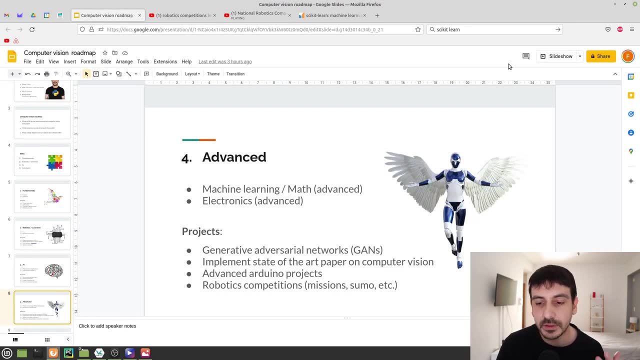 some, for example, something like this: also, some of these competitions, you are competing against other people, so the way you need to to approach problems and the way you need to build your solutions, it needs to be super robust because you are competing against other people. so if you want to develop some more advanced tools, 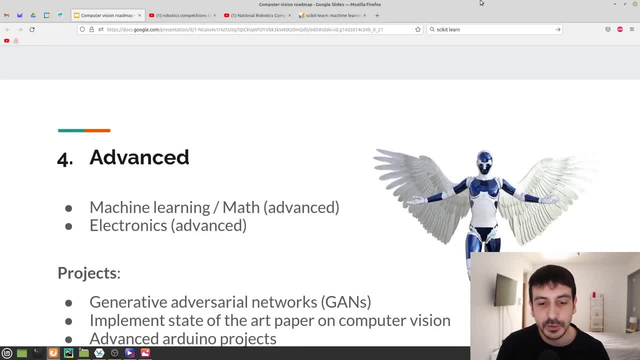 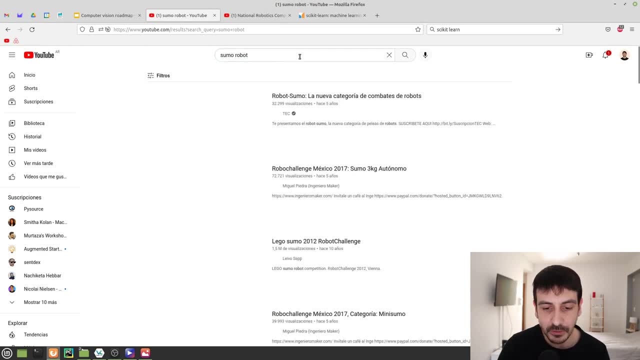 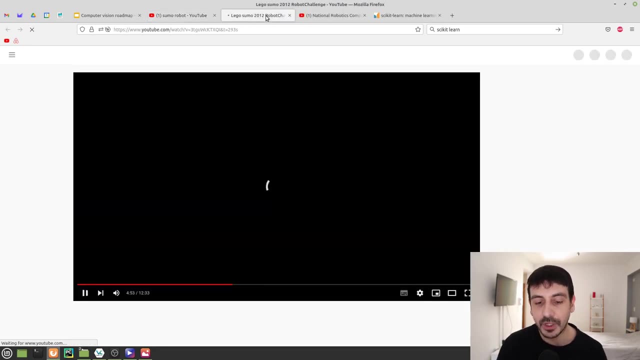 that's basically. that's pretty much a very good way to do it. also, there are some contests about sumo. let me show you. i'm not sure if you're familiar with it, but this is also a very good project in order to learn more about robotics or learn more about how, the, the, how, programming for. 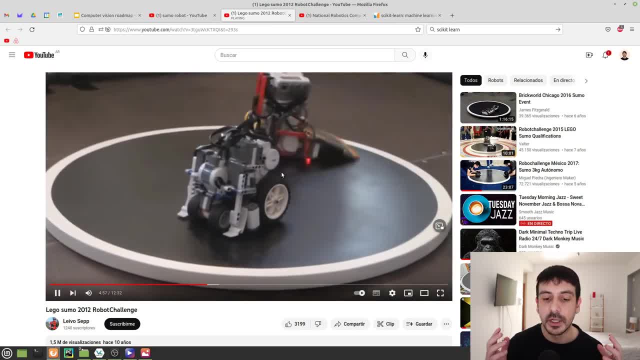 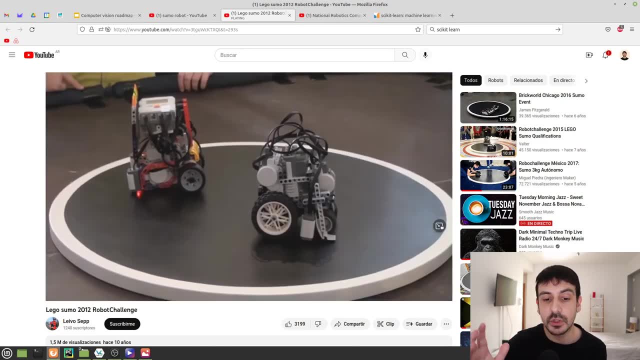 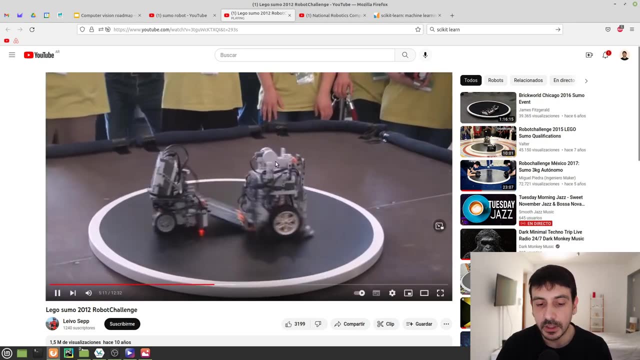 a for a physical device, for a real device, for an actual device works. remember that if you are going to work as a computer vision developer, there will be many chances, many projects in which you need to do something like real, something like physical. so you definitely need to learn how this physical 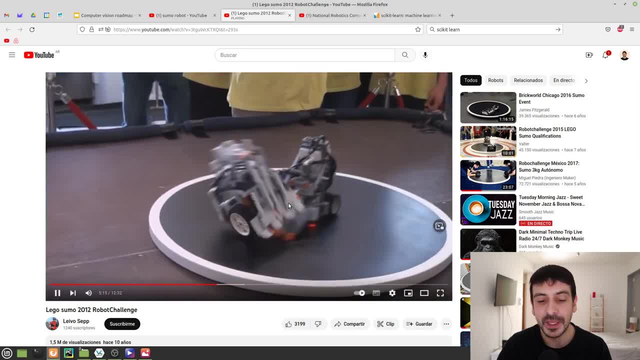 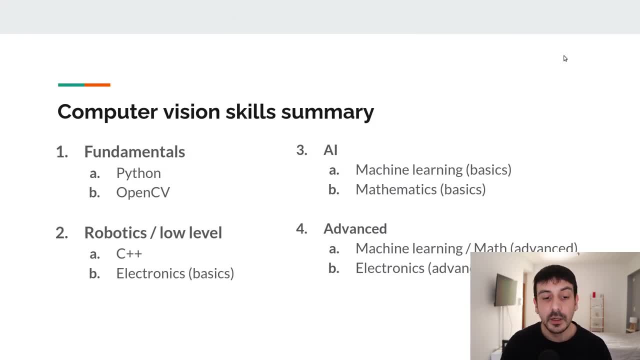 stuff works. they don't work the same way as code, so yeah, anyway, this is another project you can take in order to learn more advanced robotics. that's pretty much all the skills you need to learn in order to become a computer vision developer, or all the computer vision related skills. so this is a summary of the four modules i have mentioned. 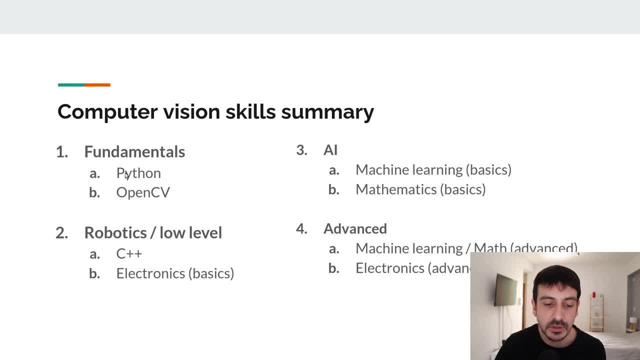 so far. basically, it's the fundamentals, the foundations, which is python, of ncb. and again, you will be surprised if you will know how many projects you can approach and you can solve by using only python and opencv. you will be surprised. this is, this is a must for every computer vision. 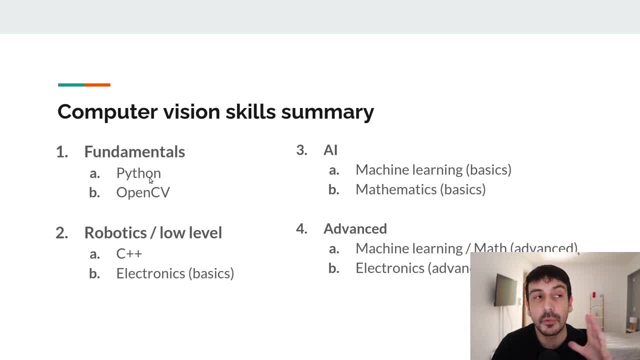 developer and by knowing python, opencv, you are going to approach maybe 70 of all available problems, so this is very important. then another module which is about robotics, or low level programming. this is where we have c++ and electronics, or the basics of electronics. then we have another model for artificial intelligence, and this is where we have 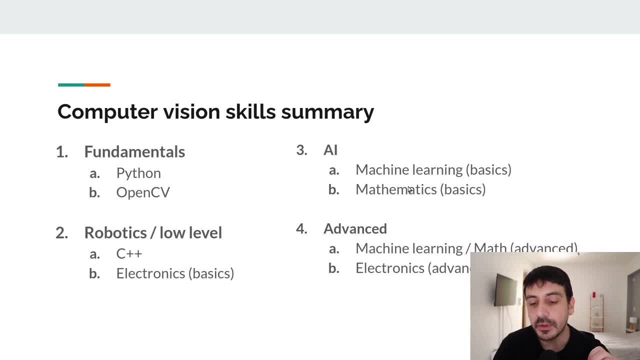 the basics of machine learning and the basics of mathematics. and then we have the advanced model, where we have the more advanced machine learning, mathematics and electronics and and, if you ask me, obviously the the first model is the most important one, and then it all depends on what do you want to do? because, for example, learning the, the low level, 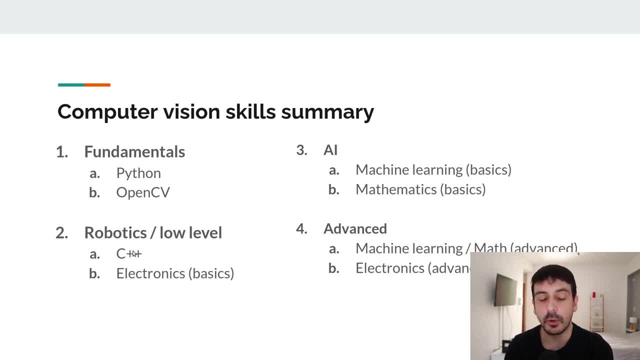 programming, learning c++ or learning how everything is, how everything works on an edge device or electronics. it's very important. it's very important, it's very convenient. it's definitely a plus. it's definitely a plus, but i will say it's not really that critical. i would say that you can. 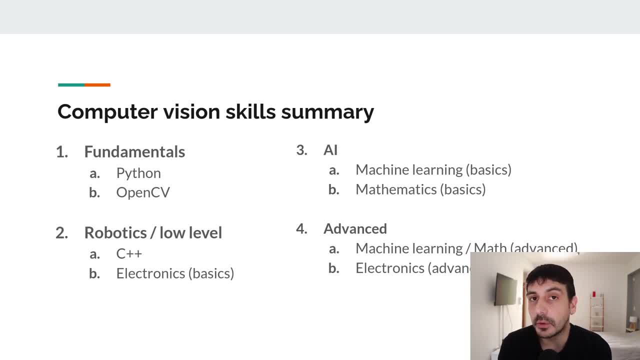 definitely work on many, many, many projects without really knowing anything about c++. you can definitely, it could definitely happen. i have worked in many, many, many, many projects which don't really involve c++ at all, so it's definitely possible. but moving on, and then the third model. 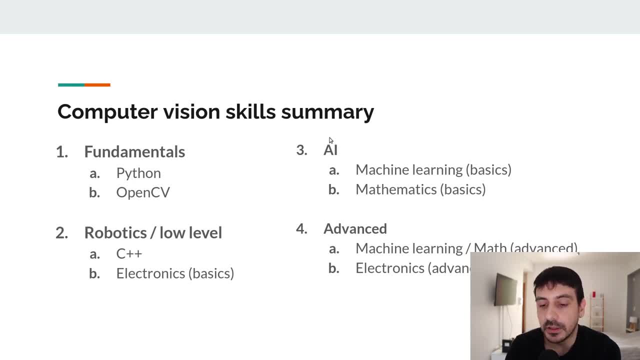 the one for artificial iterations, machine learning and mathematics. this is also very important, i will would say, if you ask me, i would say the fundamentals is the most important, and then the second one which is the most important one is the one regarding artificial intelligence. this is where 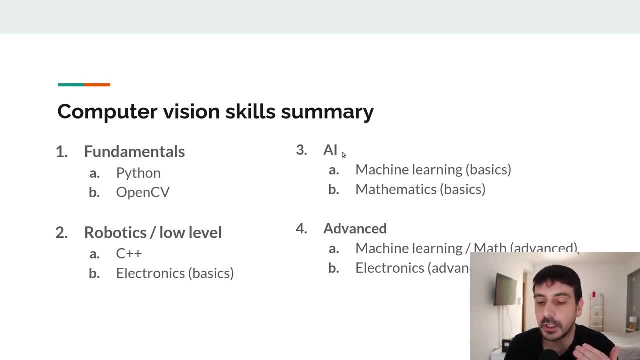 you are going to learn everything that's object detection or image classification, and all that mathematical intuition of geometries and so on. so this is definitely, definitely, definitely, very important. and then you have the more advanced module, which i'm not going to say that it's not. 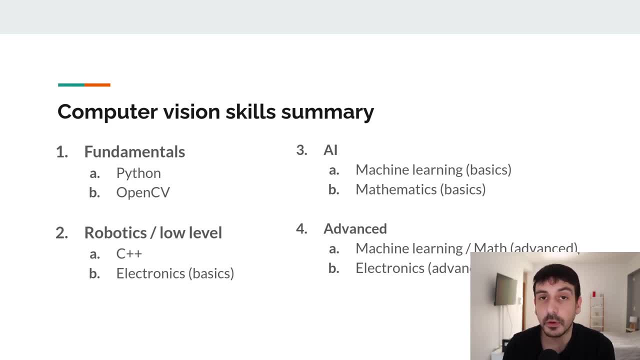 important. but i will say that if you are starting from zero, if you are starting from scratch, if you are just starting to learn computer vision, you should definitely focus on everything else. you should definitely focus on the fundamentals, for sure. then you can learn some simple plus, if that's. 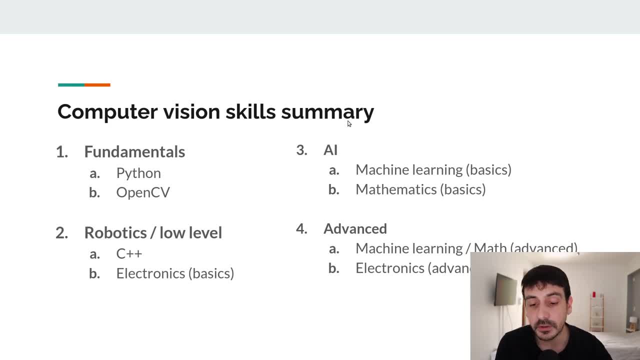 what you're into. if you want to, then you should learn some machine learnings, obviously, and then, if you want to, you can go. you can go super, super, super, super deep and learning absolutely everything there. there is to learn about machine learning or about mathematics and about electronics, but only if you have already. 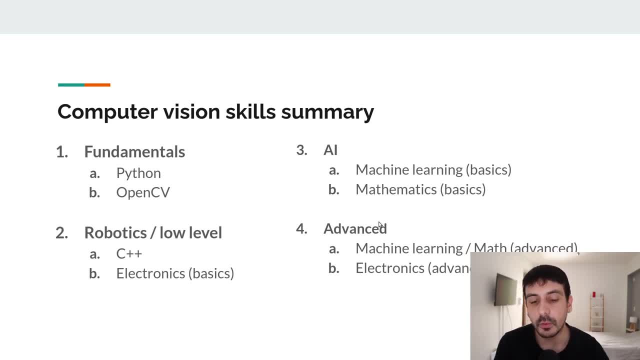 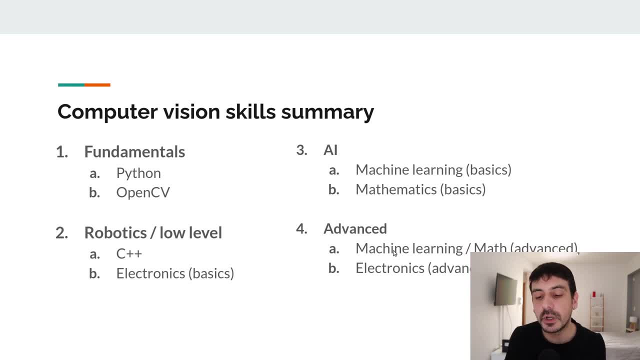 definitely learn a lot of things, and i will say that if you are starting from zero, you do it. you could be like an awesome developer and not knowing much about very, very complex mathematics. that's basically these four modules, and these are the modules which you need in order to learn the computer vision skills, but 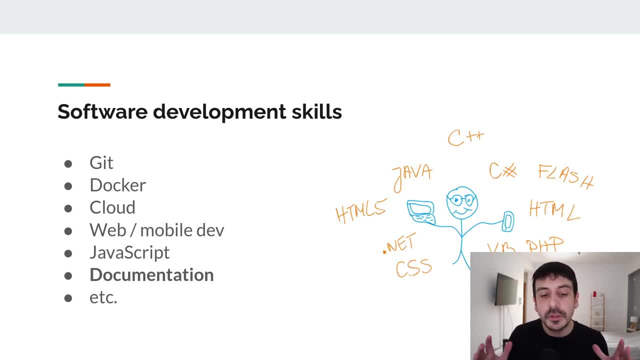 if you want to become a computer vision developer, you will definitely need to know something other than computer vision. you will need to know something other than machine learning and Python and OpenCV, and you will need to know some software, some software related skills. These are, for example, some of the 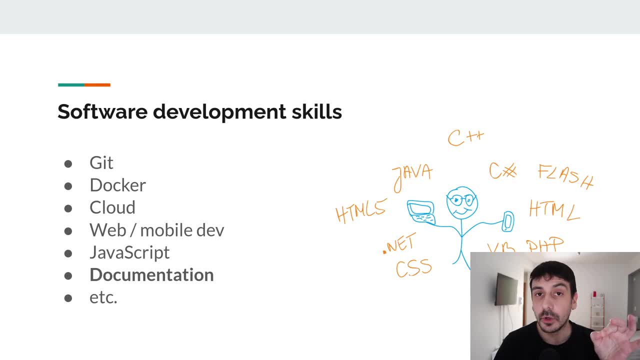 software development skills you will definitely need to know, you, you will definitely to know something about in order to become a computer vision developer, for example. some of the skills I have listed here are Git. you should definitely need to know something about Github. definitely and definitely you. 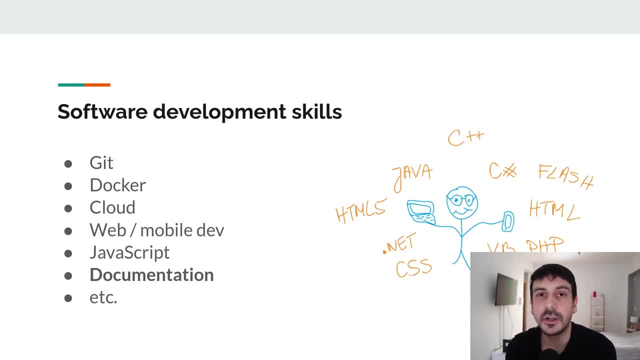 should learn, like the basic commands like git, commit and push and pull and all the basic commands that are in Github and also some of the山on libraries, the basics how to create a repository and how to clone a repository. i mean everything that's like the basics of github. but if you have the time and if you have the interest to go super, super, super. 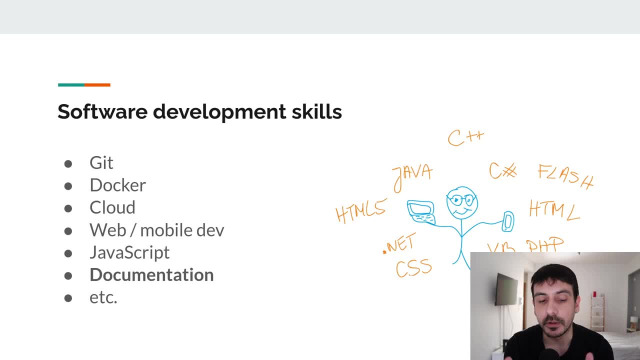 deep on github, then that's going to be much, much better. then another one which i think it's a very nice tool, a very nice software tool to learn, is docker. i will say it's not really needed to go super deep and to go super crazy with docker and to know absolutely everything there is to know. 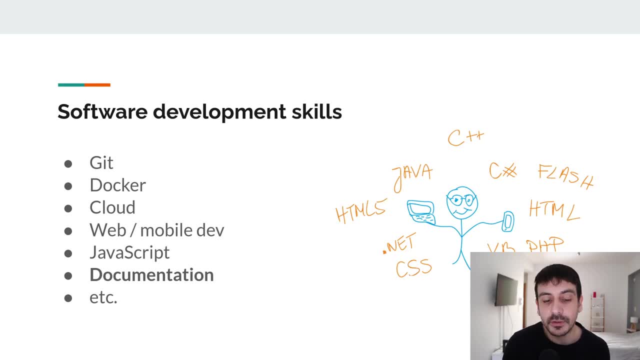 about docker, but at least, at the very least, you should know what docker is, and you should, you should understand what people say regarding dockers, what's an image, what's a container and how to how those things work. that's basically my recommendation and also the most basic docker. 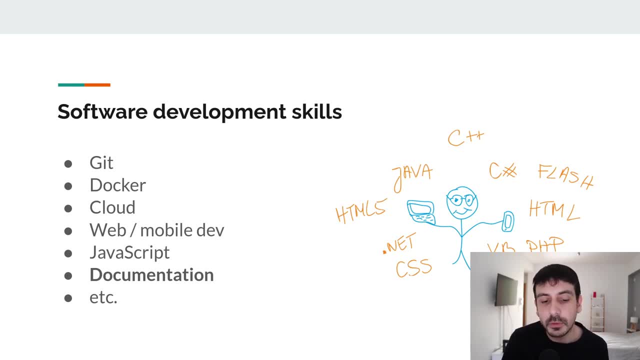 commands, the. you don't really need to go super, super deep, but at least you should have some knowledge of of what docker is and what you can do with docker. then cloud cloud providers, for example aws, google cloud or azure. this is definitely a must for a computer vision. 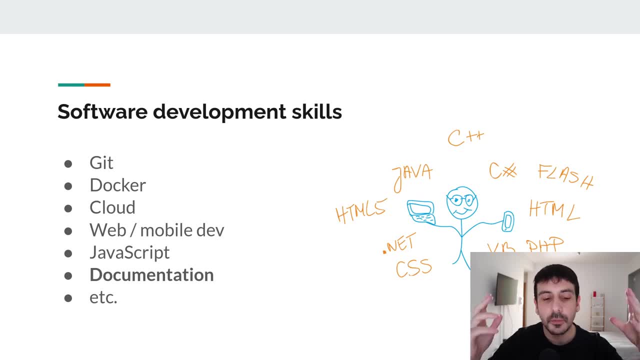 developer. there are many, many, many different services and different products in each one of these cloud providers, and the idea is basically to get familiar with all these different services and products and to know exactly what you can do in these cloud services, to know exactly what are all the different problems you can solve using these products, to know exactly how you can use. 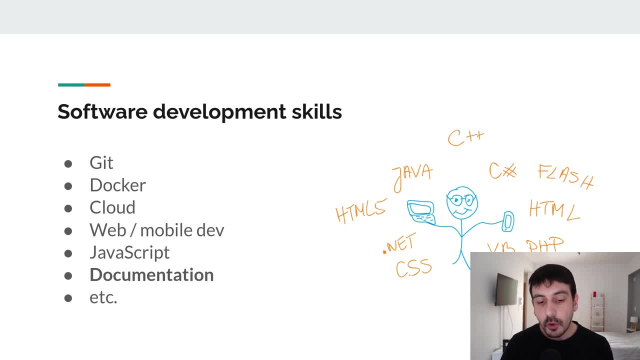 these products in order to build your solutions. then web or mobile development is another skill which is very useful for a computer vision developer. i have seen many computer vision or machine learning developers who are very fluent on web development or mobile development and it's very, very easy for them to create, for example, pocs. 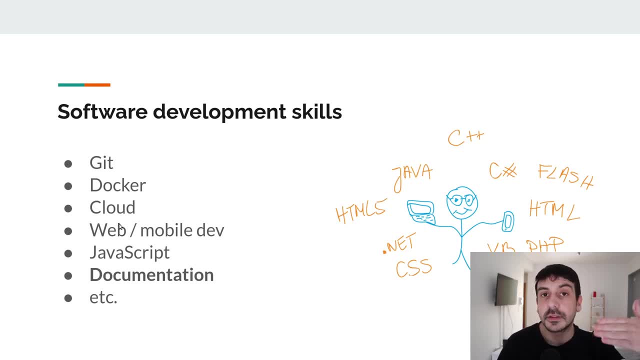 or to create like a very to show exactly their performances, how how their models perform, to make like a very visual demonstration of what they have been working on. so this is a definitely a skill. I would say it's not a must, but it's a very valuable skill then. 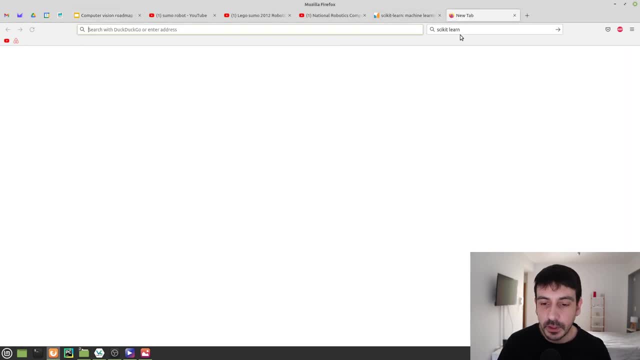 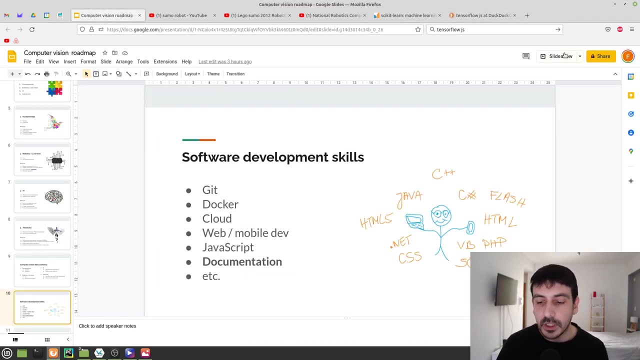 JavaScript is another example. for example, tensorflow has. if you work in, if you're working in JavaScript, you can use tensorflow GIS, which is a tensorflow library for working with JavaScript, for JavaScript developers and working as a freelancer, for example in Upwork, I have seen many, many, many different jobs which 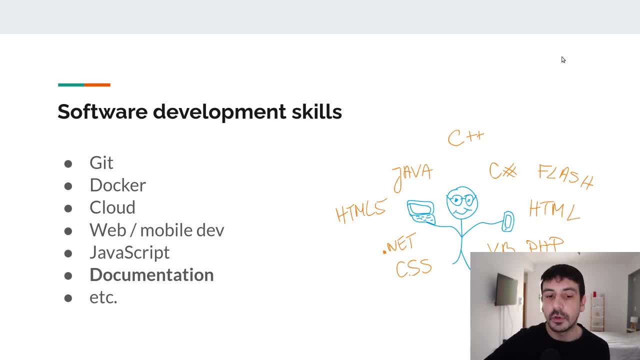 they are looking for a tensorflow JS developer. they are looking to solve a problem using tensorflow JS, so this is also definitely an important skill if you are a computer vision developer. it's not a must, but it's a nice to have, it's definitely a plus and if you are fluent in JavaScript is definitely going to be. 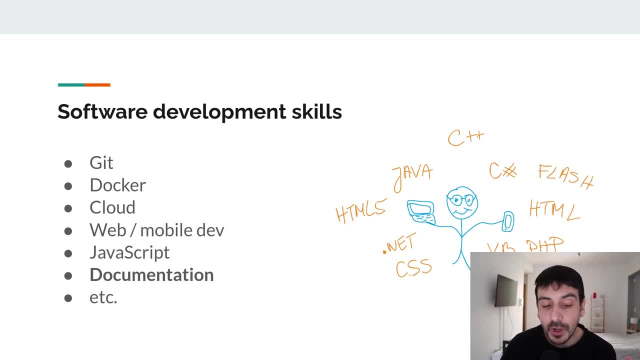 better then documentation, and there is a reason why this skill is involved, why this skill is highlighted in this list, and it's basically because I consider this is a very, very important skill for a developer, for any type of developer, and I think it's very important to become more fluent in how. 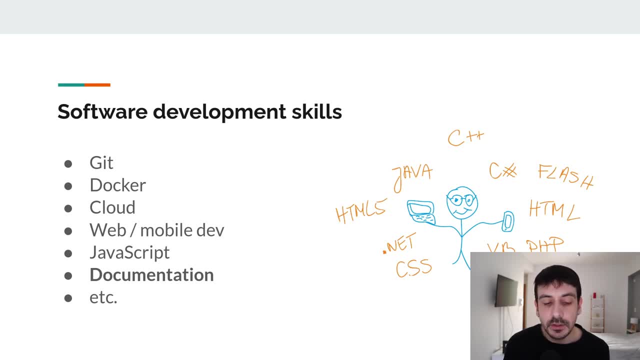 to write like a very proper documentation. this is something that many people underestimate. many people don't really focus on documentation. it's like if it's not important. but I have seen and I have experienced that it's not really trivial, it's not really simple to write like a very, very proper. 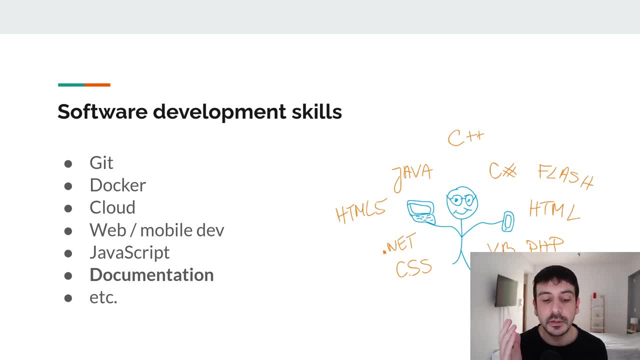 documentation. this is definitely a skill to learn over time, and there are many, many things to document for, for example. for example, a readme file in a GitHub repository, or if you work with Jira as a project management tool, you are going to have to write your stories, or you're. 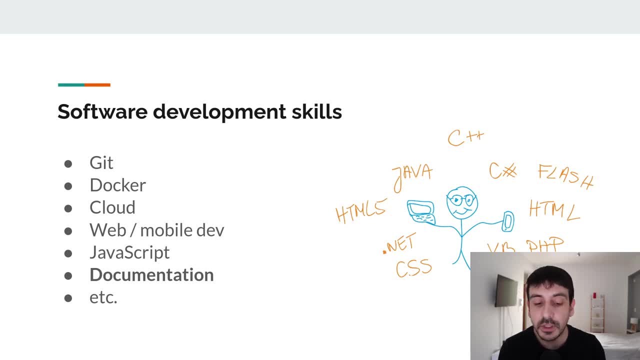 going to have to read other people's stories, so that's also another type of documentation. or if you are documenting like an entire process, like an entire pipeline, that's another type of document. so documentation is everywhere, absolutely everywhere, and it's super, super important to become more skillful on documentation. it's very important. 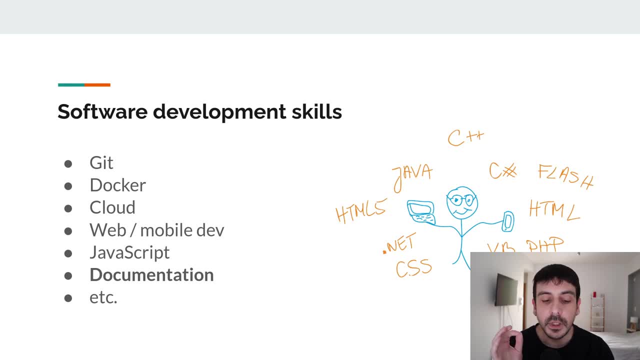 specifically if you, if you're going to work with computer vision, there will be many experiments, there will be many research that you are going to do like a lot of development, a lot of research, when you are going to be developing your models, and it's very important to document absolutely every single thing. 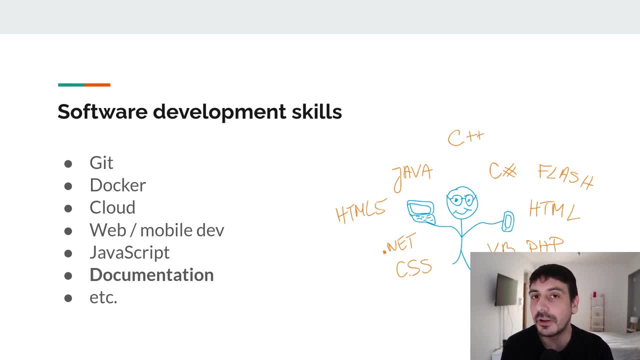 you do, because it's going to make things simpler for everyone else. so, yeah, that's why I think documentation is so important. I think it's like one of the most important skills for every developer, not only computer vision developers. and then I, you can see I have like an et cetera, because this is not a 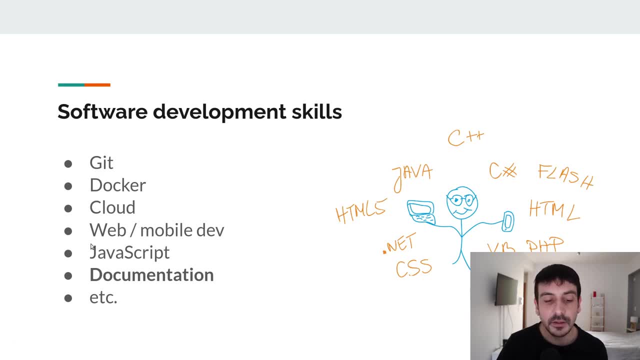 next comprehensive list. by any means. the idea is that the more software related tools you are familiar with is going to be much, much better for you. it's going to be, yeah, you're going to be a better computer vision developer, that's for sure. and as a very quick note, I can tell you that when I started working as a 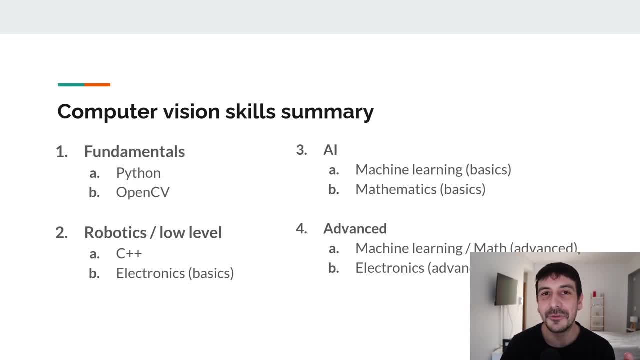 computer vision developer. I thought I was naive enough that I thought that a Python and machine learning were going to be all were going to be enough. I thought that Python, maybe some OpenCV and machine learning were going to be everything I needed in order to work with computer vision and specifically I 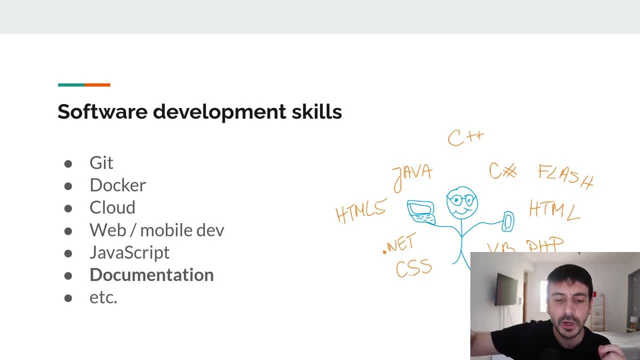 thought that everything that was like software tools or software related was completely unimportant. that was what I thought, and boy I was wrong. boy, I was super, super, super, super, super, super wrong. and over time I realized how important is to get more familiar with all the different software related tools. 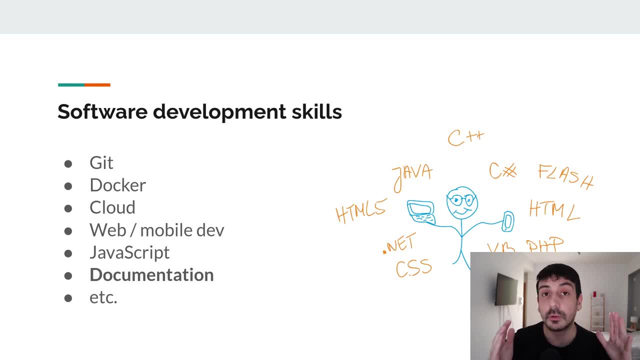 different programming languages, absolutely everything you can learn is going to be much, much, much better, much better. so yeah, it's always about not inventing the wheel right. there are many problems which have already been solved, and it's always like a good idea to to get familiar with all the solutions. 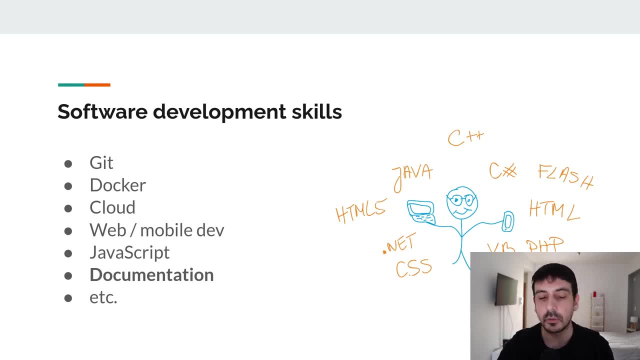 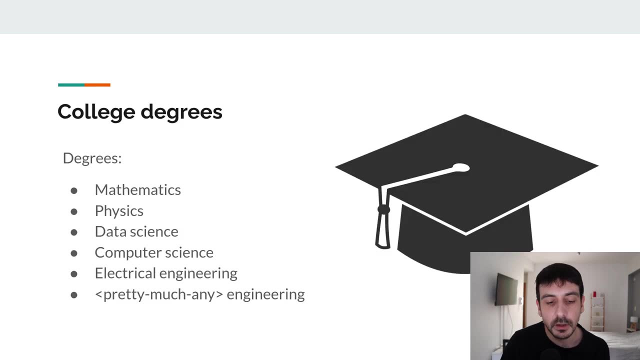 available, because it's going to be much easier for you to just create new solutions or to approach new projects. if you like, have like a good background of everything that's already available. but anyway, now let's continue with the college degrees. so far i have mentioned all the skills. 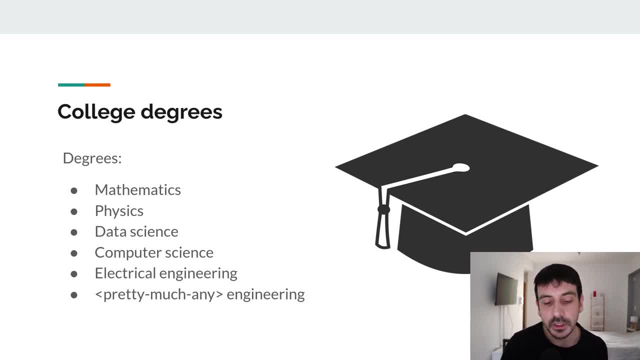 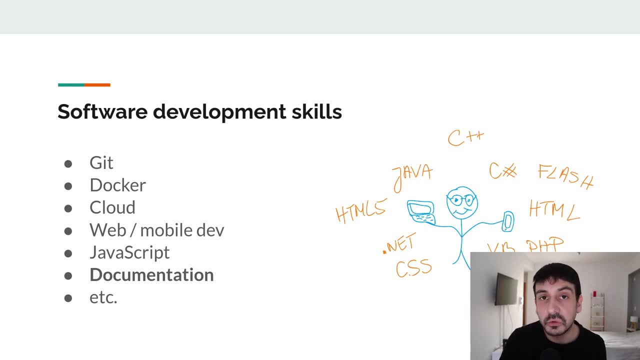 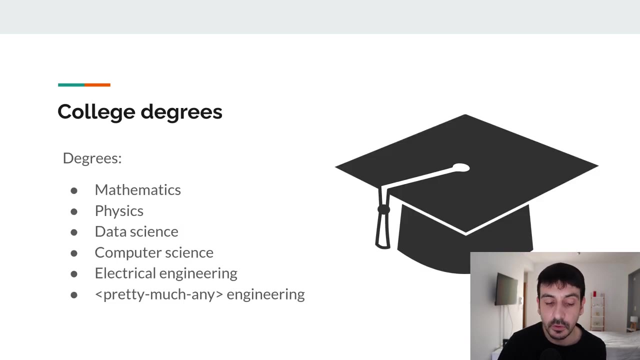 you should learn in order to become a computer vision developer. and you can perfectly approach any of these skills, of everything i have just mentioned, by your own, by taking projects, by taking youtube tutorials or by taking online courses, by working on your own. definitely, you can learn absolutely everything i have mentioned so far. but if you would like to take a college, 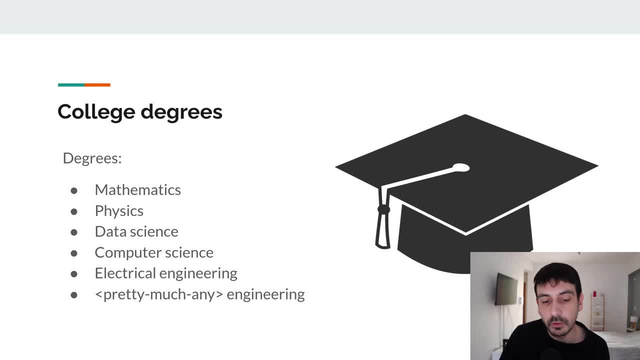 degree, if that's what you like, because there are people who prefer college degrees and that's perfectly valid. these are some of the college degrees that i think it's. they are going to give you the foundations to learn everything we have just mentioned in this video. it could be a college. 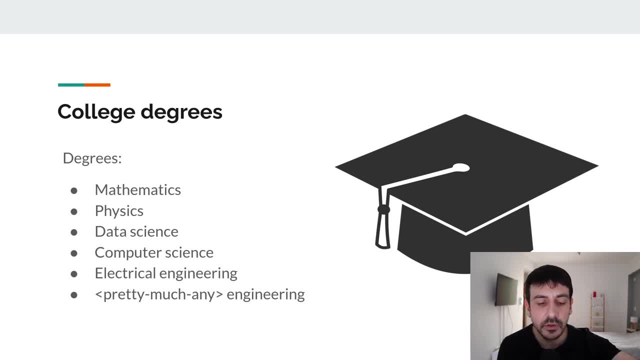 degree in mathematics, physics, data science, computer science, electrical engineering or pretty much any engineering, absolutely every single one of these degrees will give you the way to approach problems, the way to think about problems, the way to come up with solutions, and that's pretty much what's the most. 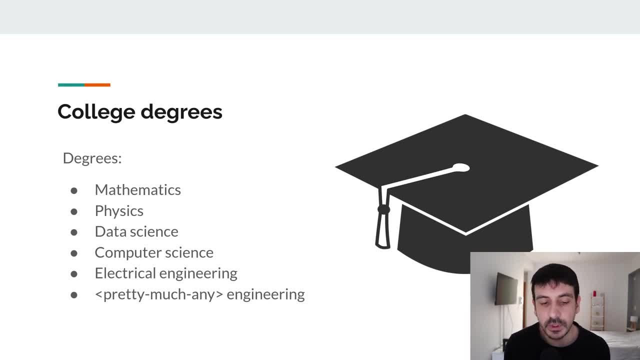 important thing then it's just taking a few courses and learning python, opencv and so on, but again, this is only a way to learn all of these skills or learn like the way you should approach problems, but this is perfectly possible to learn everything that you need to know. 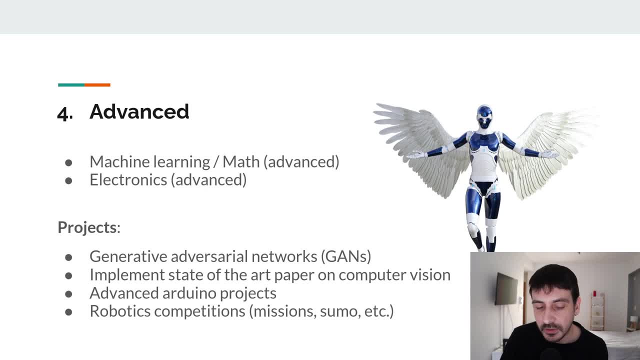 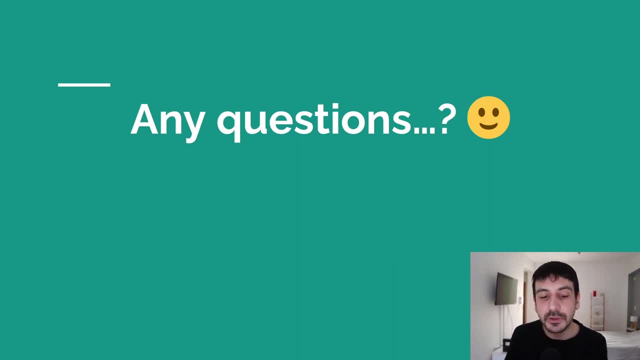 everything on your own by taking projects and by taking courses and so on. it's perfectly, perfectly possible. so this is going to be all for this computer vision roadmap, and then please let me know if you have any questions, because if you do have any questions, just write me a message in the. 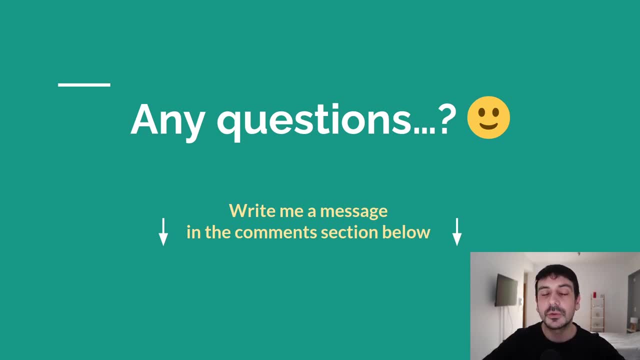 comments section below and i will be super, super, super happy to answer absolutely every single question you may have about absolutely everything i have just mentioned in this video. so if you have any question, please write me a message in the comment section below. that's going to be all for.